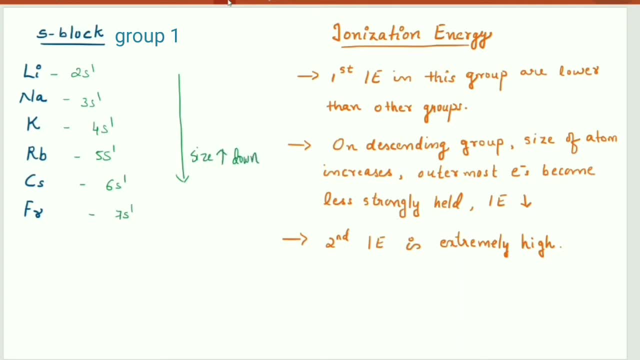 Size increases down the group. So cesium is more big. So cesium is more big than rubidium, potassium, sodium, lithium. So size increases down the group. So ionization energy. So what is ionization energy? The energy required to remove the outer electron. So first, ionization energy in this group are lower than compared to other group. 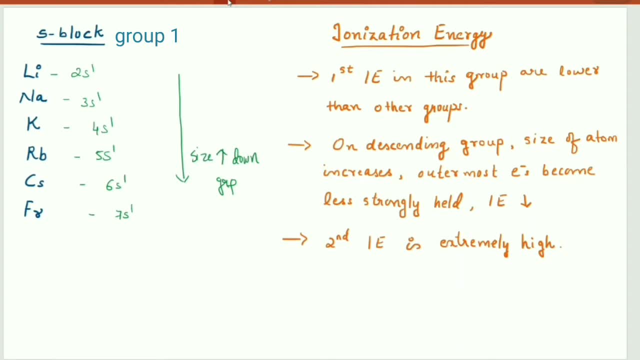 So alkali metals, that is S block elements. first, ionization energy is lower than other group. Descending group size of atom increases. Outermost electrons become less strongly held. Ionization energy decreases. So on descending group size of atom increases. So size of atom is increasing. So that means the shell is increasing. 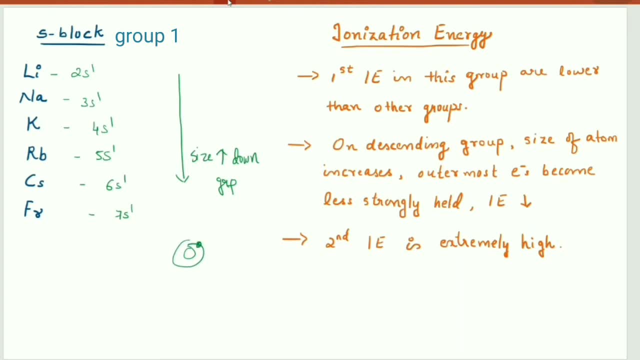 So the outermost electron is loosely bound, loosely held, So it is very easy to remove this electron. So if it is loosely held, then it is easy to remove. It is easy to remove this electron, So the ionization energy is low. Ionization energy will be low. 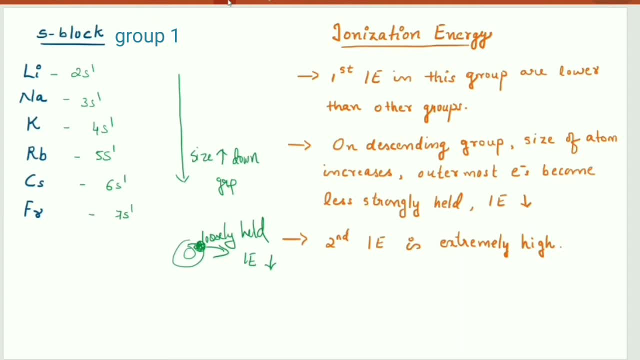 And second, ionization energy is extremely high For cesium. what is the electronic configuration? Outer electronic configuration: 5P66S1.. So when first, ionization energy means the electron from cis S1 is removed, This electron is removed. So now the outer electronic configuration 5P66S1. 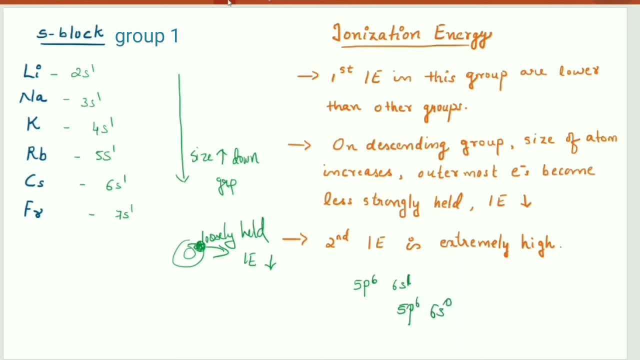 So next second ionization energy means we have to remove another electron from 5P6. So 5P6 is completely filled. So it is very difficult to remove the electron from 5P6. Since it is completely filled or half filled, the ionization energy will be greater. 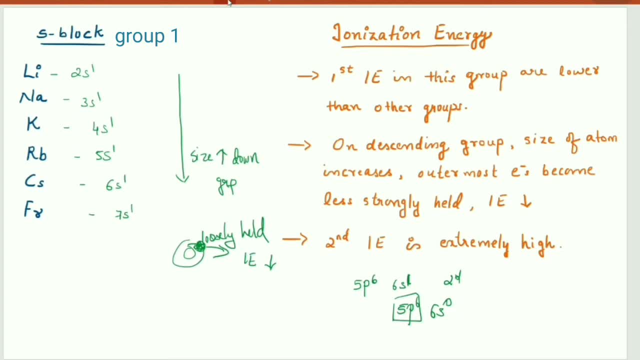 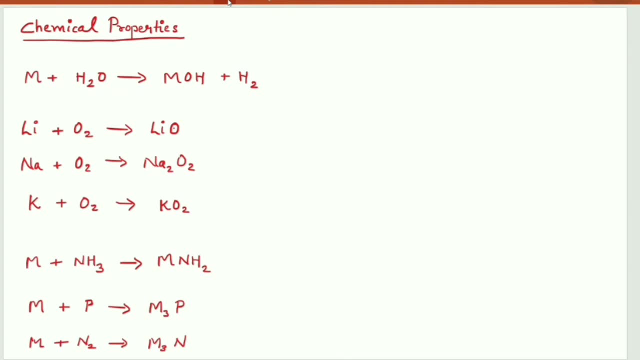 So second, ionization energy is extremely high for alkali metals. Now coming to chemical properties: M plus H2O- alkali metal, M for alkali metal, any alkali metal, lithium, sodium, potassium, etc. So M plus H2O give MOH plus H2O. 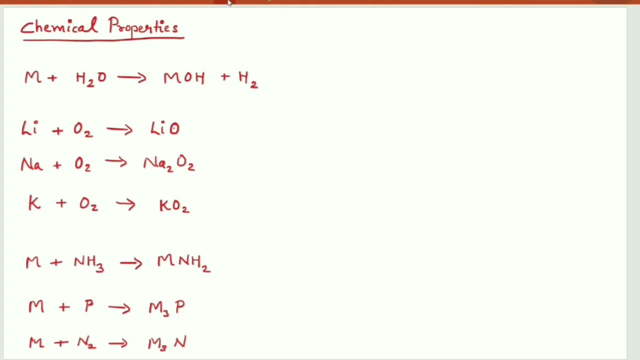 So hydroxides are strongest bases, So hydroxides are formed with alkali metals. Hydroxides are formed And lithium plus oxygen give LiO, It is a monoxide. And sodium plus O2 give Na2O2.. It is a peroxide. 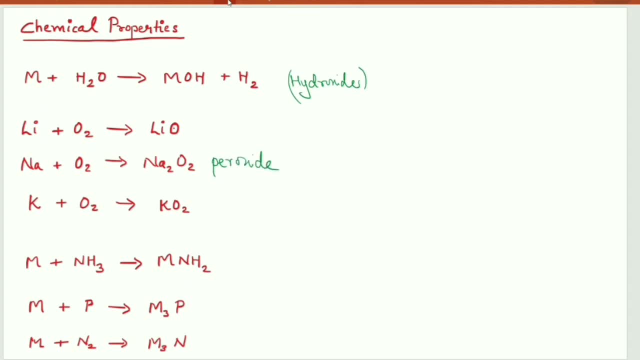 So sodium plus oxygen give Na2O2 peroxide. K plus O2 give KO2.. KO2 is a superoxide, So peroxide, superoxide, monoxide are formed Monoxide. Next M plus NH3.. So metal with ammonia give MNH2.. 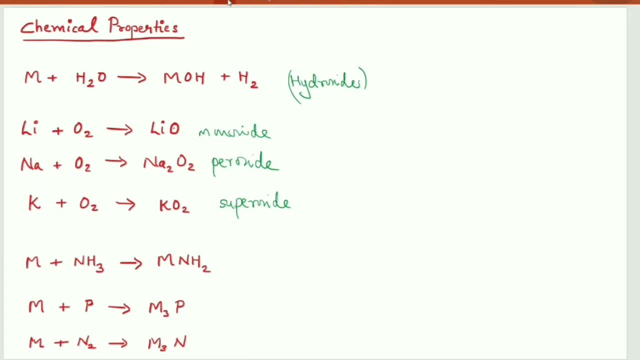 So amines is formed. Amides are formed, So M plus NH3, MNH2.. Then M plus phosphorus. So with phosphorus, what is formed? M3P? It is phosphide. So phosphides are formed using alkali metals. 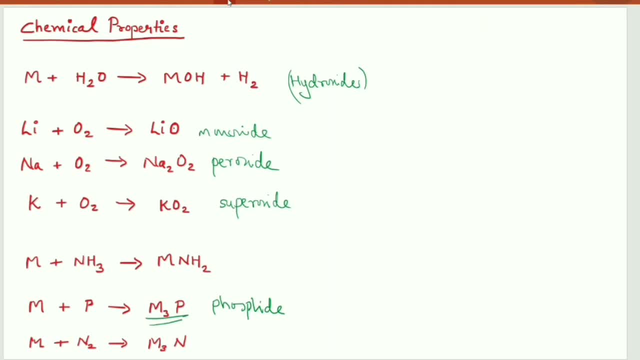 M plus M2.. M3N, So nitrites are also formed. Then phosphoroxide monoxide hydroxides are formed. Next is sodium bicarbonate: NaH3O2.. Na2CO3.. It is sodium bicarbonate. 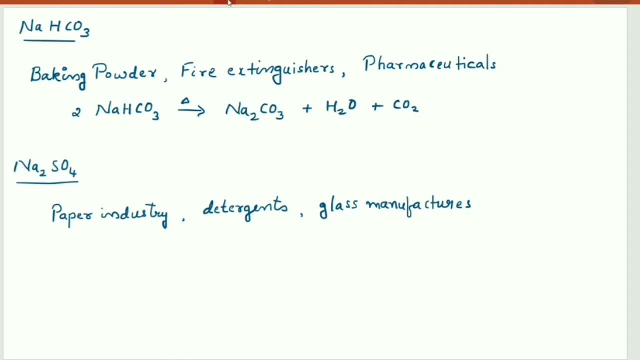 So it is used as baking powder in fire extinguishers, in pharmaceuticals etc. 2- NaHCO3 in presence of heat: Na2CO3 plus H2O plus CO2.. So the reaction of sodium bicarbonate with heat is it gives sodium carbonate plus water, plus carbon dioxide. 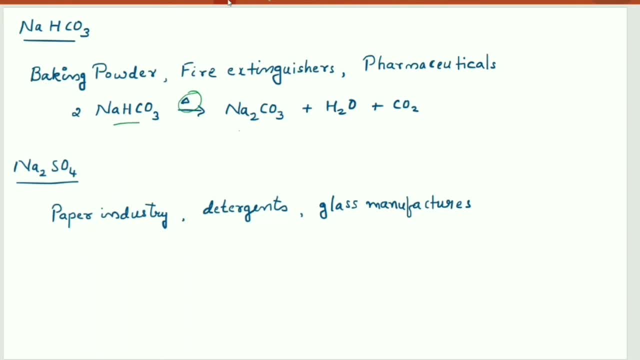 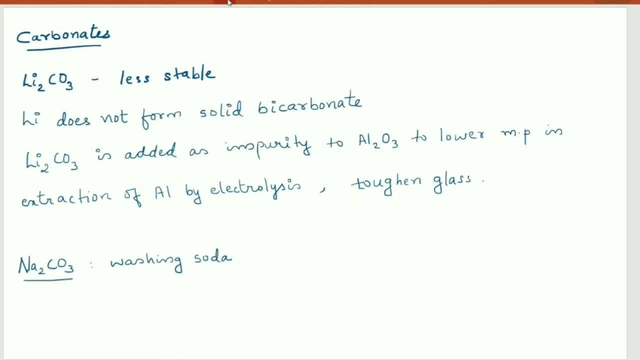 And next is sodium sulfate And it is used in paper industry, Detergents, glass manufacturers. Next is carbonates: Lithium carbonate. It is less stable. Lithium carbonate is less stable, So alkali metals can form carbonates, hydroxides, oxides, peroxides, bicarbonates, etc. 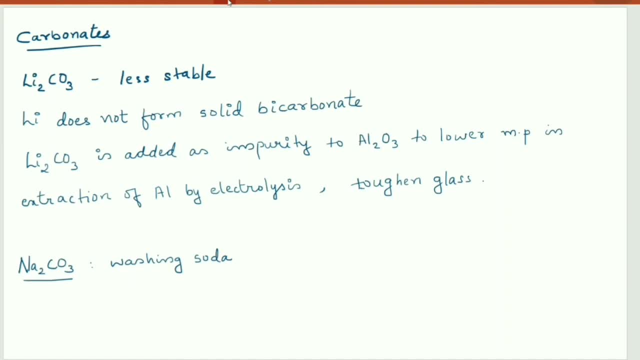 And lithium does not form solid bicarbonate. To be noted, lithium does not form solid bicarbonate But it can form bicarbonate in solution form. Lithium carbonate is added as impurity to aluminium oxide to lower melting point in extraction of aluminium by electrolysis. 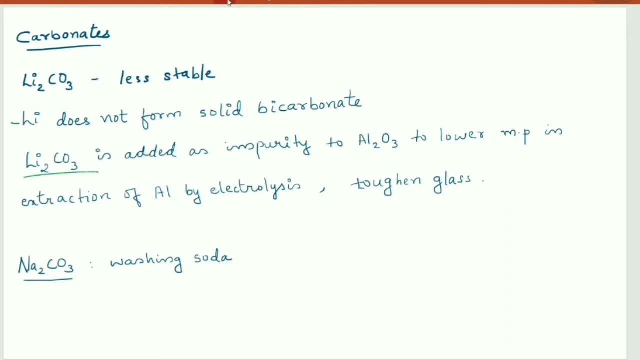 So lithium carbonate is added as impurity to aluminium oxide in the process of extraction of aluminium, And another use is it is toughened glass. It is used for toughening the glass And sodium carbonate is used as washing soda. Sodium carbonate is used as washing soda. 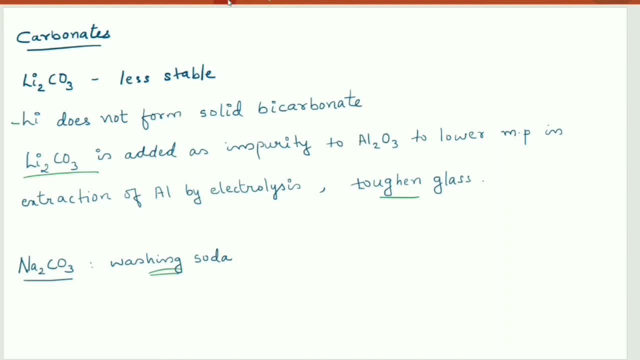 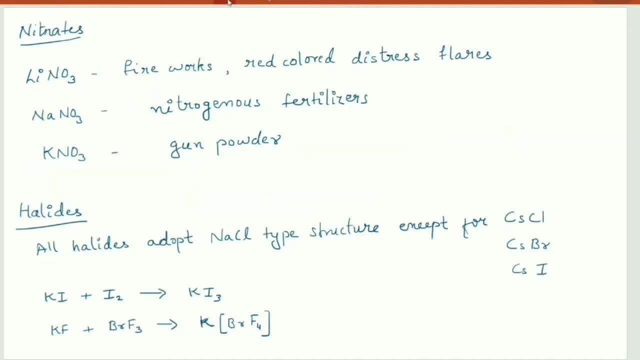 And sodium bicarbonate is used as baking powder. So sodium bicarbonate is used as baking powder And sodium carbonate is used as washing. Another compounds formed by alkali metals are nitrates, So LiNO3.. Nitrate- Lithium nitrate. 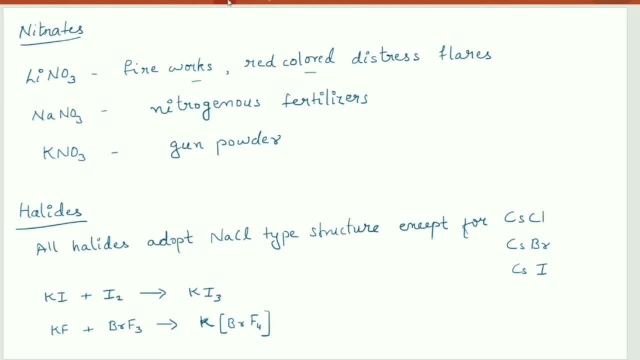 It is used in fireworks- Red colored distress flares. So in fireworks, what is the element contained? LiNO3.. Lithium nitrate And NaNO3 is used as nitrogenous fertilizers In fertilizers. NaNO3 is used as gun powder. 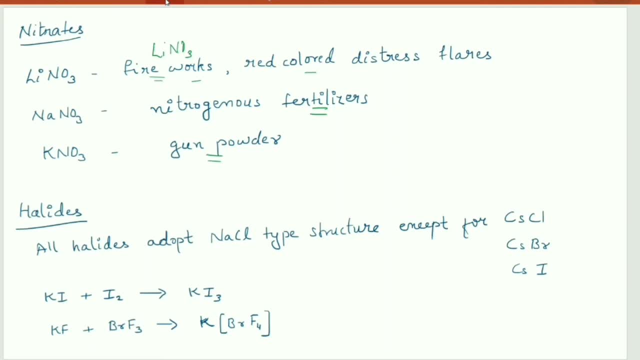 So NaNO3 is used as gun powder. Next is halides. All halides adopt any Cl type structure except for cesium chloride, cesium bromide, cesium iodide. Just look on this reaction: Ki plus I2.. K. potassium iodide plus a halide I2.. 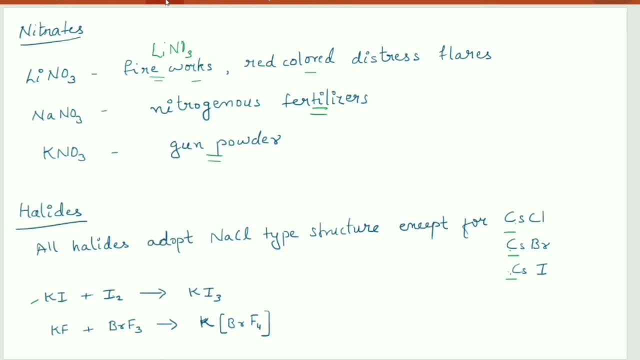 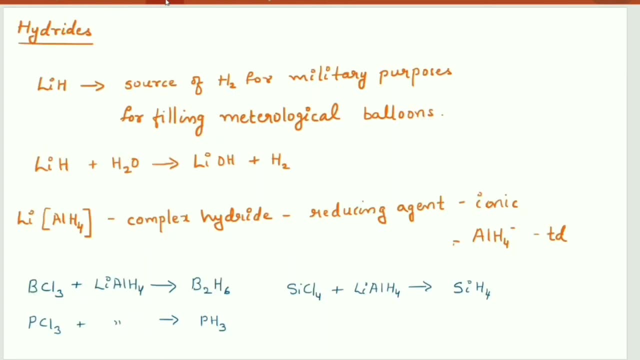 Give Ki3.. And KF plus BrF3.. Give KBrF4.. This is hydride LiH, Lithium hydride, Source of hydrogen for military purposes, for filling meteorological balloons, And lithium hydride plus water. 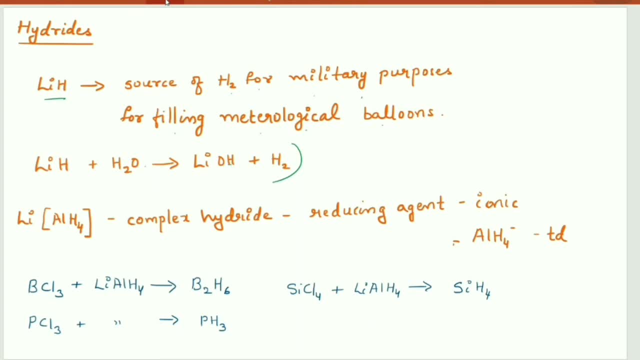 Give lithium hydroxide plus H2.. Lithium hydride is reacted with water to form lithium hydroxide, And another type of hydride is lithium aluminium hydride. It is a complex hydride And it is a reducing agent. 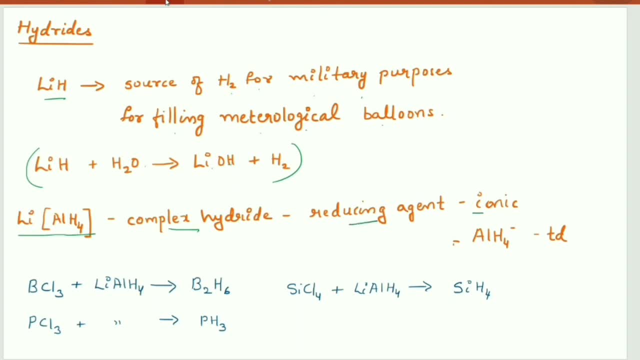 And it is ionic. So how it is ionic: AlH4 minus is ionic In ionic form And it is in tetrahedral shape. And reactions of lithium aluminium hydride are given here: BCl3 plus lithium aluminium hydride. 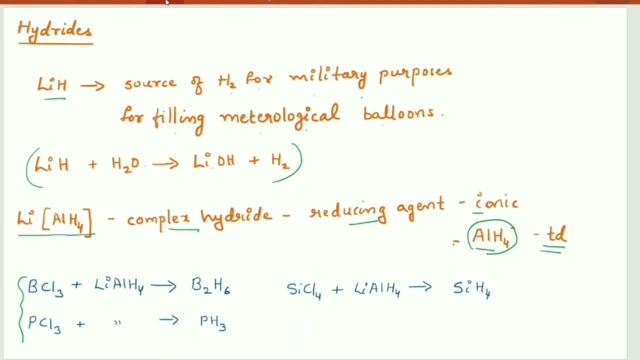 Give B2. Which is borane And SiCl4 plus LiAlH4.. Lithium aluminium hydride, Give SiH4.. Silane, And next is with PCl3.. So it will give Ph3, that is phosphane. 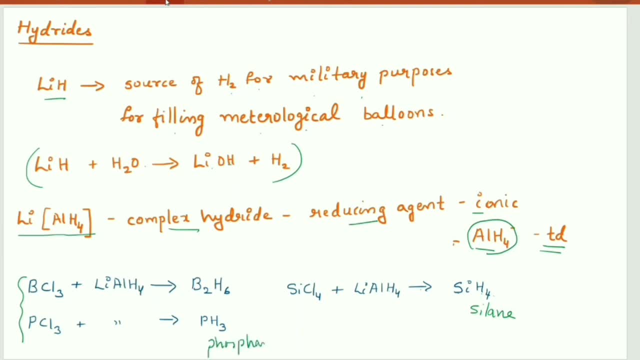 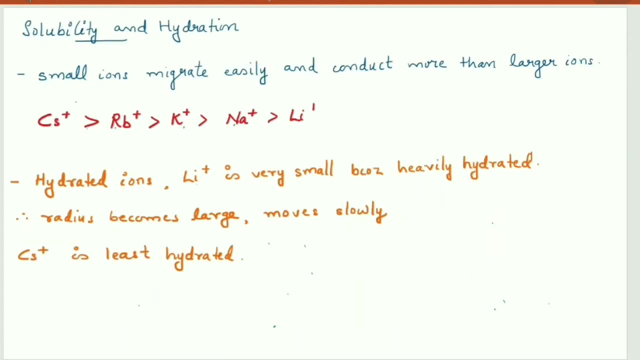 So phosphane is formed when PCl3 is added with lithium aluminium hydride. This is a powerful reducing agent. Next we can discuss about solubility and hydration. So the important point to remember is small ions migrate easily and conduct more than larger ions. 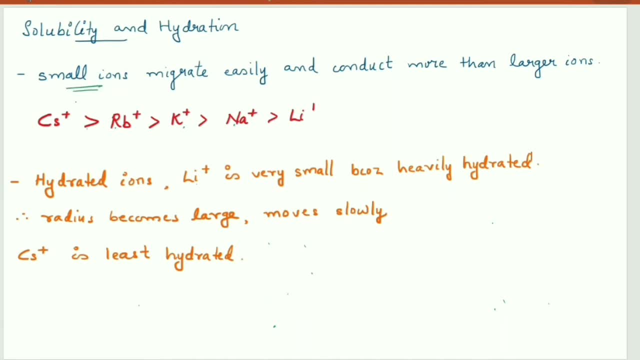 Smaller ions can move faster And migrate easily and conduct more than larger ions. So what is small ion? lithium, Sodium, Potassium, Rubidium, Caesium. So among this, which is smaller, lithium is smaller. Lithium is smaller. 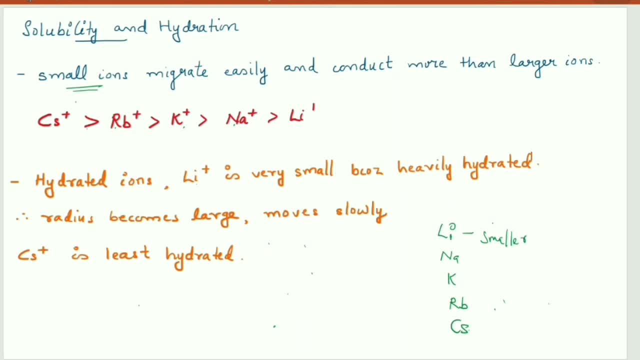 Lithium atom is smaller When coming to the ions in aqueous solution. So in aqueous solution what happen? The lithium is smaller, So lithium can accommodate H2O water molecule easily or more, So more H2O molecule is accommodated in lithium atom. 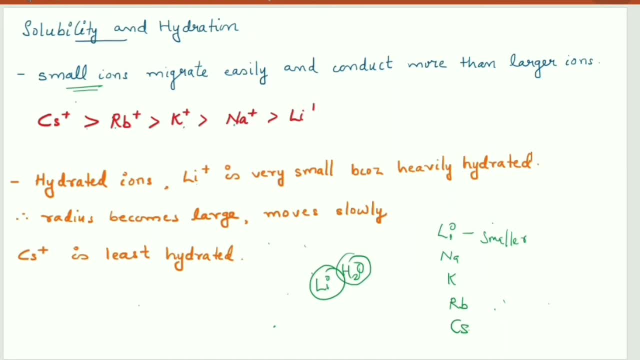 Because of its smaller sizes. So what happen? The radius of the molecule become larger, So the radius become larger. So when the radius become larger, The molecule is larger, So it will move slowly, So Li+, Li+ Will move slowly. 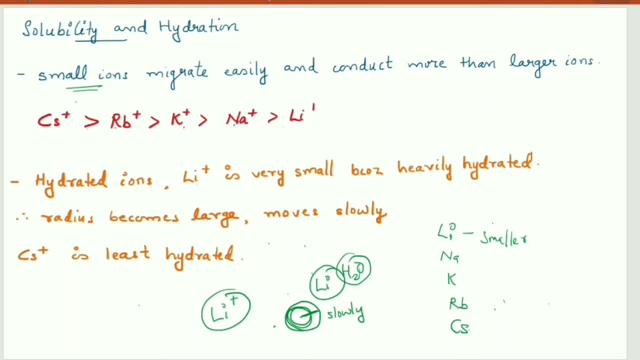 So the solubility order of the ions are Caesium+, Rubidium+, Potassium+ Sodium+ Lithium. Why Li+? Ok, The point is hydrated ions. Li+ Is very small because heavily hydrated Radius becomes large. 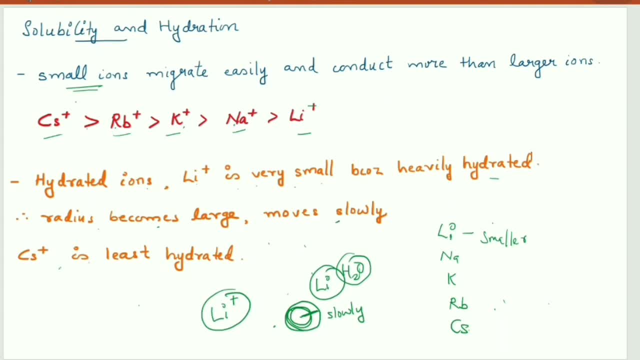 Move slowly. Caesium+ Is least hydrated, So the hydration order is reverse. Caesium+ Is least hydrated, So it can move easily. So it will conduct more than lithium, Caesium, Rubidium, Potassium, Sodium, Lithium. 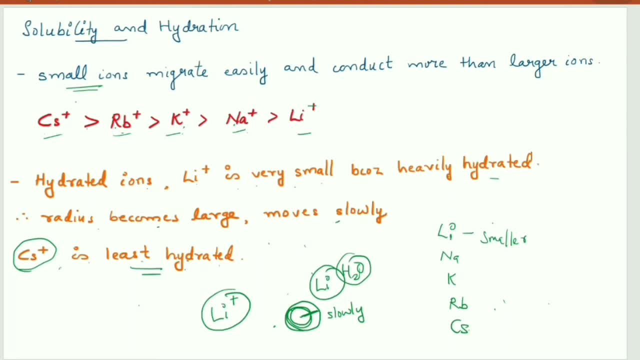 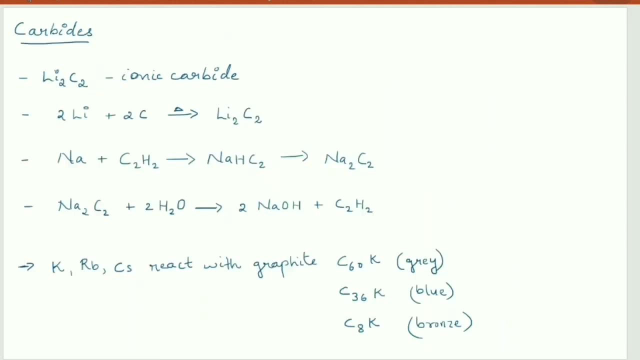 Is the order of solubility? And for hydration, what happen? Caesium ion is least hydrated And lithium ion is highly hydrated. So due to high hydration of lithium ion, It have solubility low, Conductance low. Another type of compound formed by alkali metals are carbide. 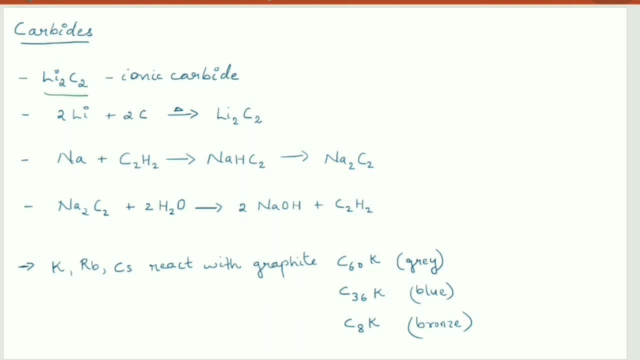 So what is carbide? Li2C2.. Lithium carbide, It is a ionic carbide And the reaction how it is formed: 2 lithium plus 2 carbon. when heated Lithium carbide is formed, Then sodium plus C2H2 give NaHC2.. 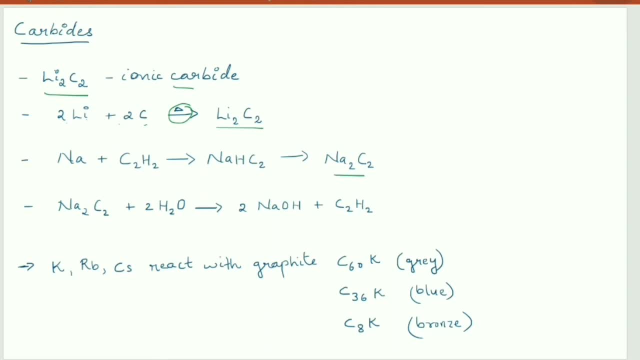 And then Na2C2.. So only for lithium. it is easily formed, Easily formed by heating. Carbide is formed easily by heating. For sodium and potassium they are undergoing some other steps also. Sodium plus C2H2 ethylene. First sodium is reacted with ethylene. 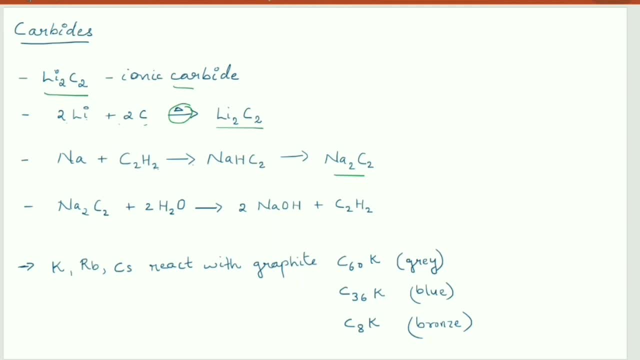 Then sodium bicarbide is formed, Then sodium carbide, Then Na2C2 plus 2H2O. Sodium carbide plus water give sodium hydroxide And potassium rubidium caesium. react with graphite C60K. It is a gray compound. 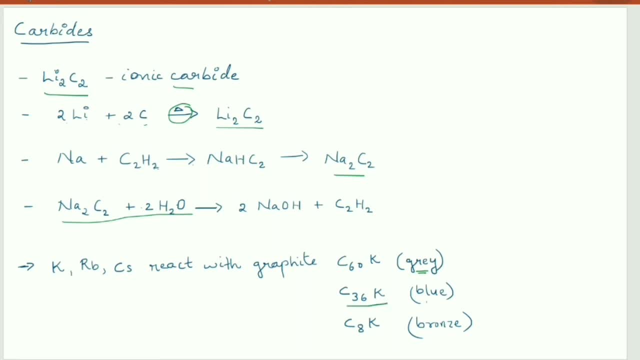 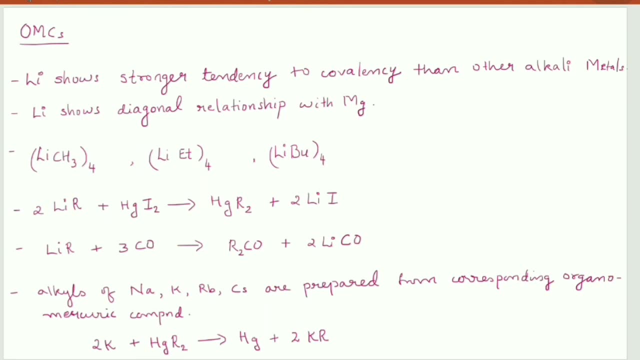 Then C36K blue compound, C8K is bronze color. Next we can see some organometallic compounds formed by alkali metals. So first, lithium shows stronger tendency to cobalency than other alkali metals. Lithium shows diagonal relationship with magnesium. 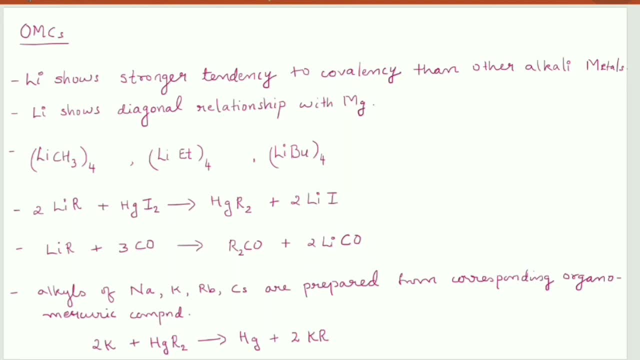 So when lithium is showing diagonal relationship with magnesium, The properties magnesium, The properties that are shown by magnesium, will also be seen in lithium. So lithium can form like Brignard reagent etc. So LiCH3 4 times, LiEt 4 times. 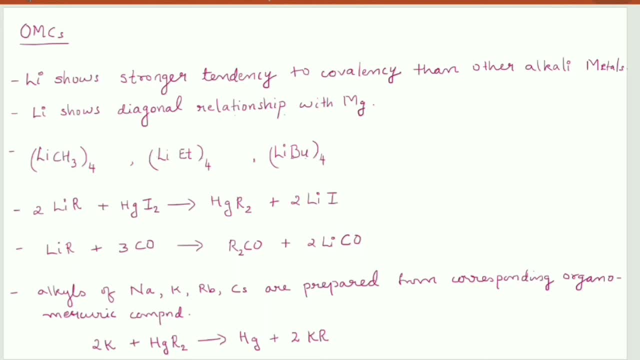 LiBu 4 times are formed. And just remember this reaction: 2LiR alkyl lithium plus HgI2 mercuric iodide give HgR2 plus 2Li iodide, Lithium iodide And LiR alkali. 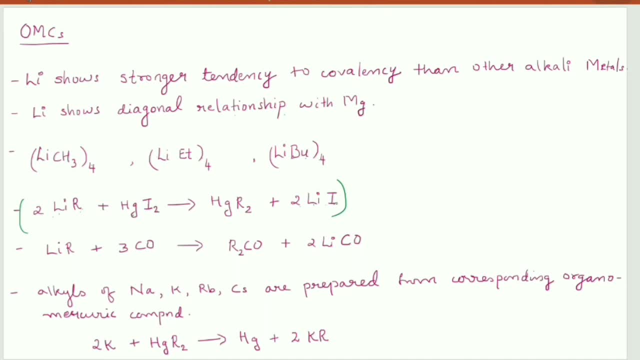 And LiR- alkyl lithium plus 3Cu- give R2Cu plus 2LiCu. R2Cu is a ketone, So ketone is formed. when alkyl lithium and 3C carbon monoxide is reacted, Ketone is formed. 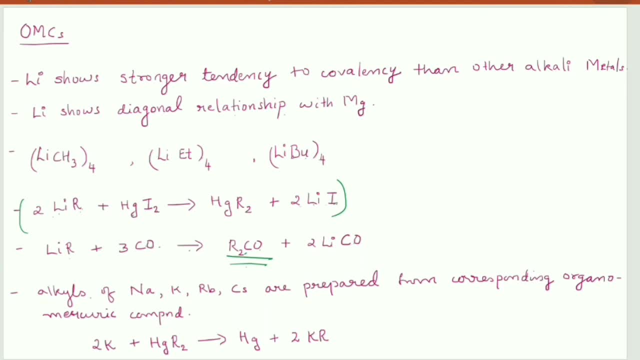 Then alkyls of sodium, potassium, rubidium, caesium are prepared from corresponding organomeric compound. So alkyls of sodium, potassium, rubidium, caesium can also be prepared like lithium, And 2K plus HgR2 gives Hg plus 2KR. 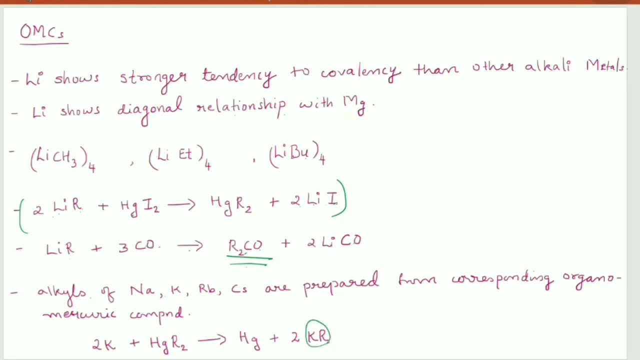 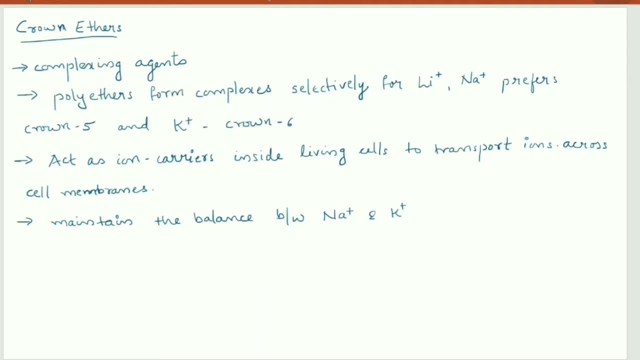 Like alkyl lithium. alkyl potassium is formed- 2KR- from HgR2 mercuric compound. Another important point is crown ethers. So crown ether is a complexing agent. So the structure of crown ether is like this: O, O and 2 oxygen atom will be there. 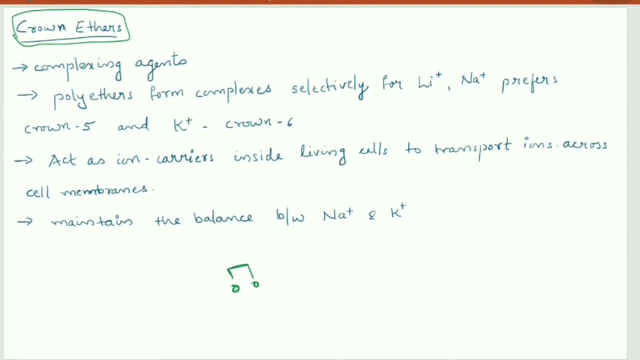 And it is connected by 3 bonds, Then O O, then again bond, Then O, O and okay. So here how many oxygen is present: 1, 2, 3, 4, 5. 5 oxygen is present And how many single bonds. 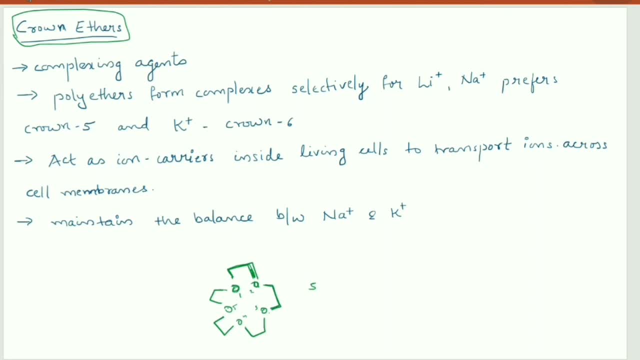 1, 2, 3, 4, 5, 6, 7, 8, 9, 10.. 10, 11, 12, 13, 14, 15.. So how to name this crown ether? This is the structure of a crown ether. 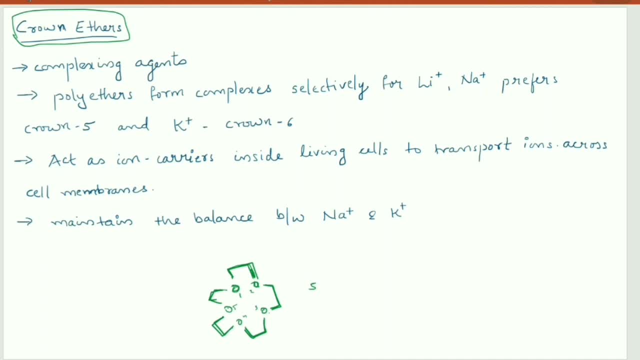 So we have to name this crown ether. So we will name this crown ether using the number of single bonds and the number of rings and the number of oxygen atom. So how to name? 15 single bonds are present, So 15 crown and number of oxygen atom: 5.. 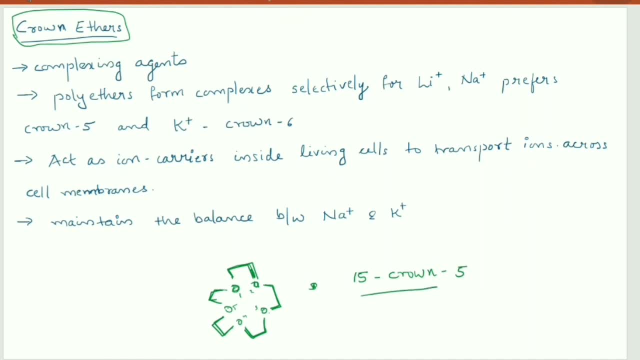 So the name of this crown ether is 15, crown 5.. So what? this is used in alkali metals. So these are complexing agents And these poly ethers form complexes. selectively for lithium sodium and prefer crown 5 and for potassium, crown 6.. That means on the cavity. On the cavity, that is this position. A lithium atom can be Encapsulated, or sodium atom or potassium atom can be encapsulated, So act as ion carriers inside living cells to transport ions across cell membrane. So the main function of crown ethers is it act as ion carrier. 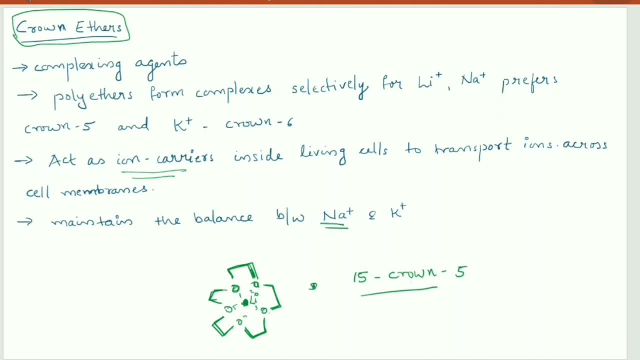 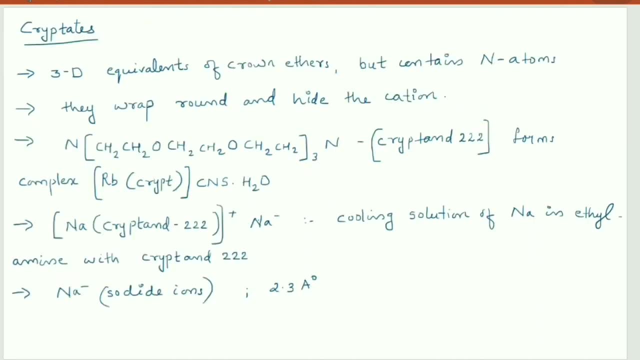 So it maintain the balance between sodium and potassium in our cell. Next category is cryptid. So what is cryptid? It is just like crown ethers, and one difference is it contain nitrogen atom. So it is 3D, 3 dimensional equivalent of crown ethers, but contain nitrogen atom. 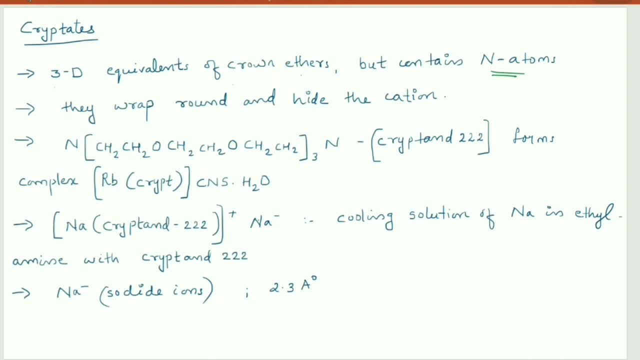 They wrap round and hide the cation. So it is hiding the cation And one of the general cryptent is N, that is, nitrogen, CH2CH2O, CH2CH2O, CH2CH2, thrice N. So cryptin 2: 2- 2 is the name for this. 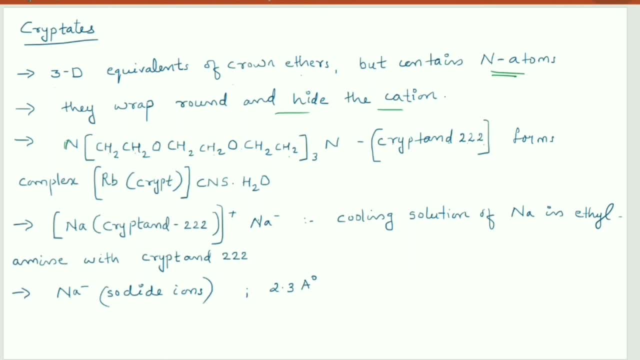 And it forms complex rubidium cryptin: CNSH2O. So another complex. And this complex is important. I will tell you why. Because sodium cryptin 2, 2 plus N A minus. So in this compound, what is the speciality? N A minus. 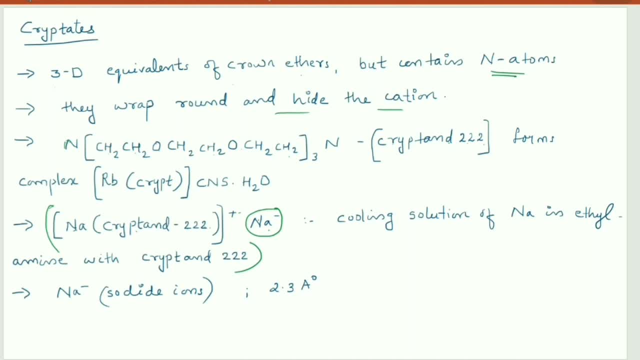 N A minus is formed here. So it is formed by cooling solution of sodium In ethylamine with cryptin 2, 2, 2.. So N A minus is formed in this complex. So just remember this. And the radius is 2.3 angstrom for N A minus. 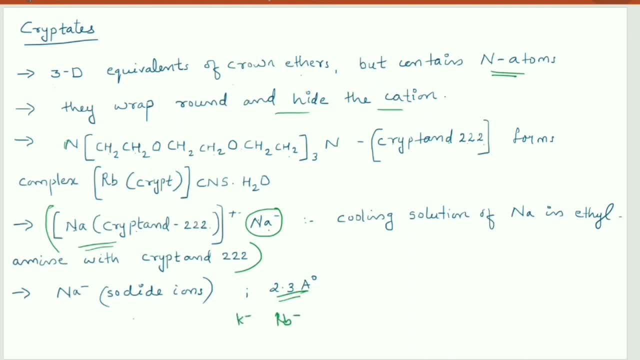 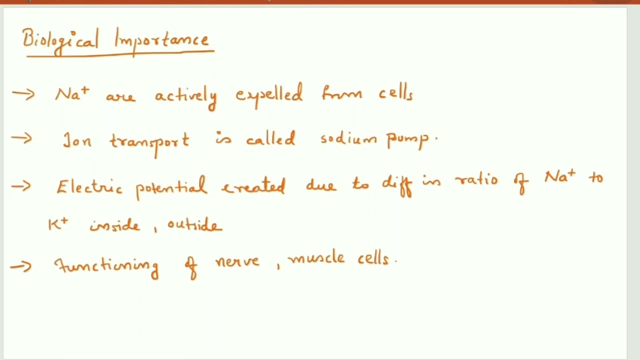 So K minus R, B minus ions are also formed. So this have to remember: N? A minus iodide is formed, 2.3 angstrom And biological importance of the alkali metal is what N A plus are actively expelled from cells, So sodium. 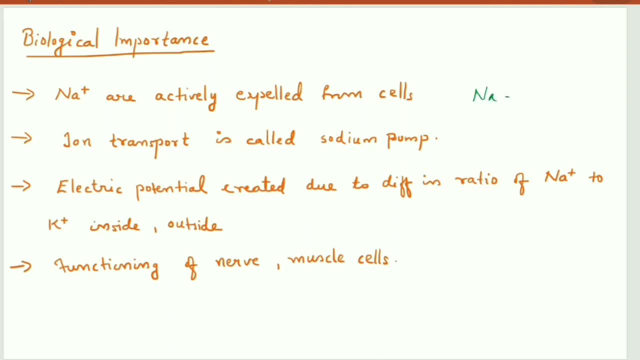 Sodium is expelled, Sodium is out and potassium, N, A plus is out and K plus is in. So sodium ions are expelled from cells And potassium is intake, And ion transport is called sodium pump. So this transportation of ions, That is, out and in of sodium and potassium, 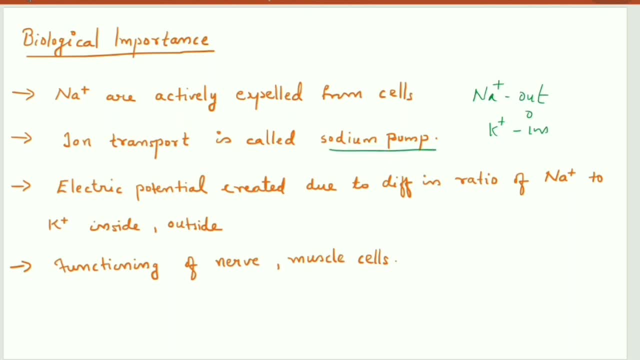 And potassium is called sodium pump. Electric potential created due to difference in ratio of N A plus to K plus inside, outside, is used for functioning nerve and muscle cells. So the electric potential, So when transportation of ions happen, a potential, A potential will be formed. 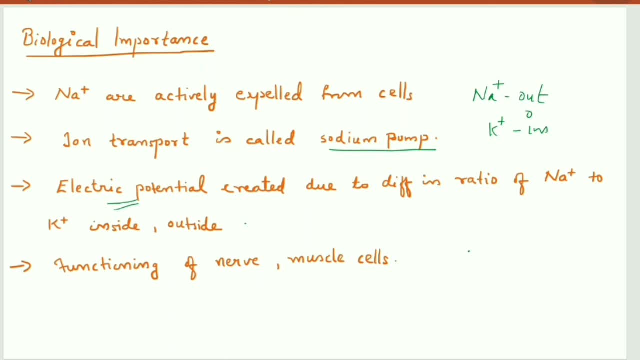 And that potential is helping the functioning of nerve and muscle cells. So for functions of nerve and muscle cells This electric potential caused by sodium pump is used. So that is the main biological importance of alkali metal, sodium and potassium.